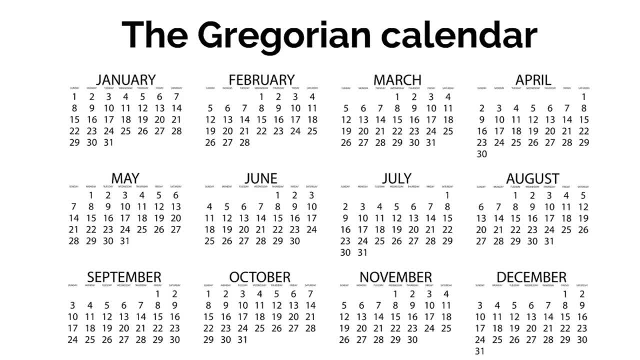 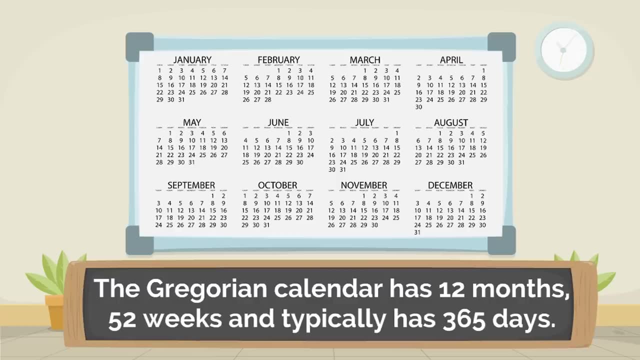 Uh-huh, Gregorian calendar. The Gregorian calendar is probably the calendar that is used in your classroom or in your home right now. The Gregorian calendar has 12 months, 52 weeks and typically has 365 days. Notice, we said typically because there are leap years. 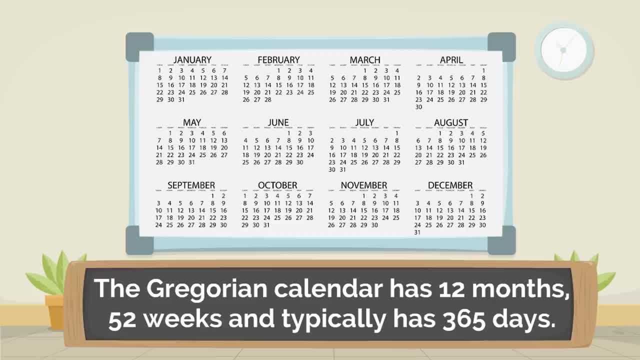 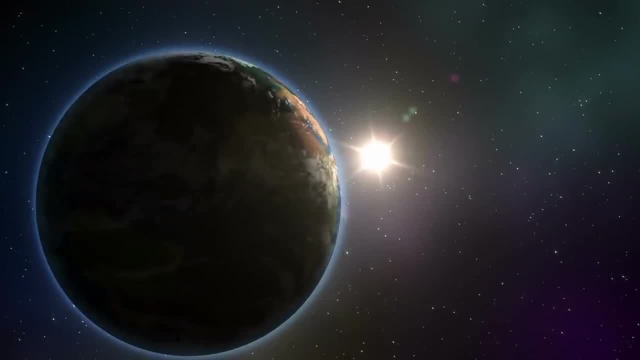 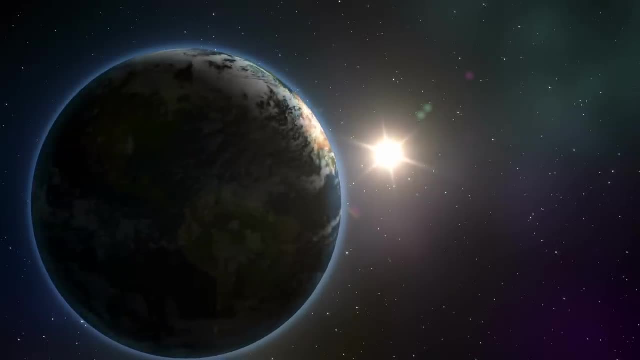 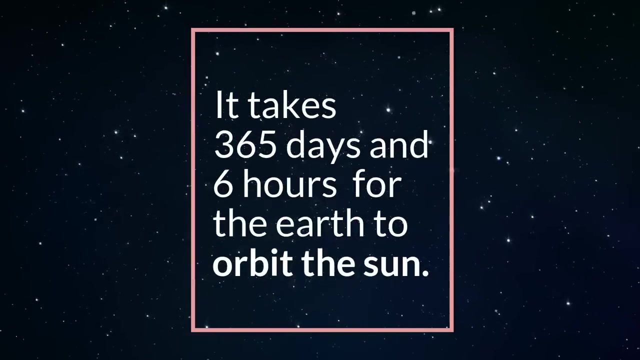 and leap years are years that have an extra day, but usually 365 days. It's interesting With the Gregorian calendar: the length of a year is based on how long it takes the Earth to completely orbit the Sun. It takes 365 days and 6 hours for the Earth to orbit the Sun. 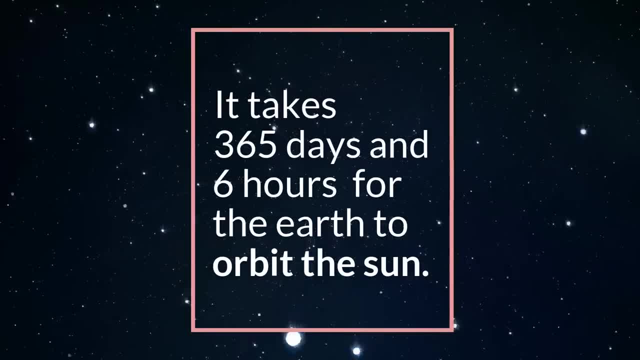 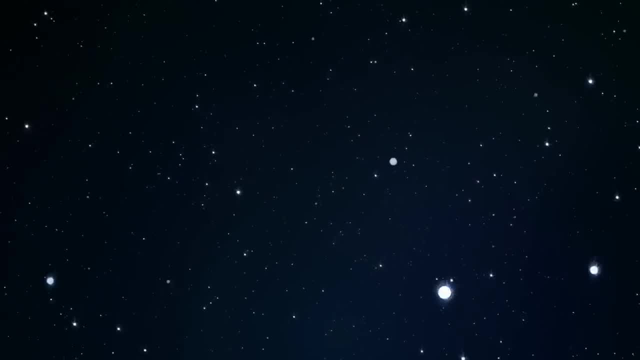 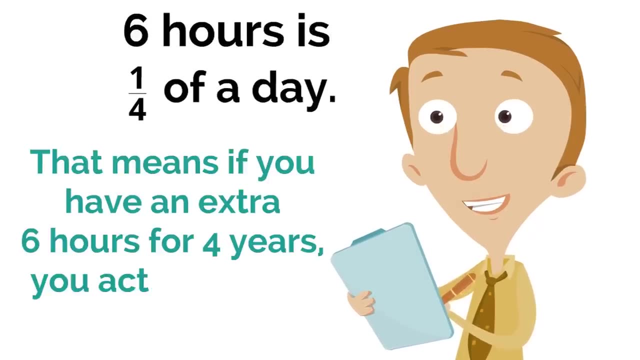 And that's the problem. It doesn't take exactly 365 days. Those extra 6 hours each year add up 6 hours is one-fourth of a day. That means if you have an extra 6 hours for 4 years, 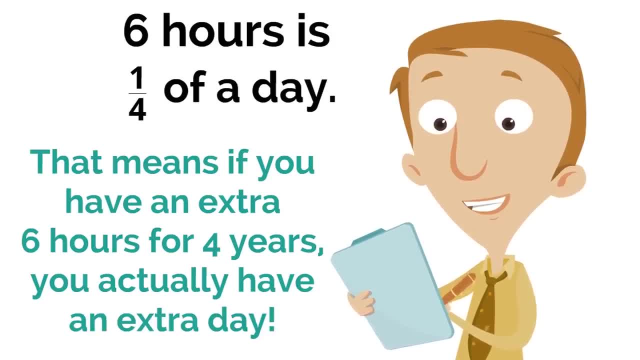 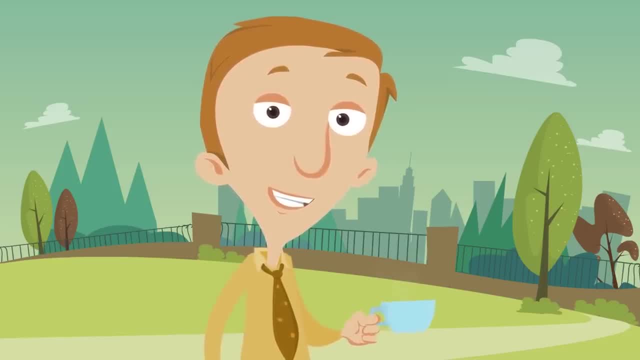 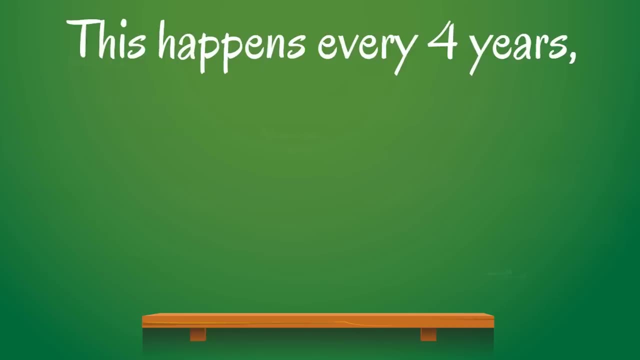 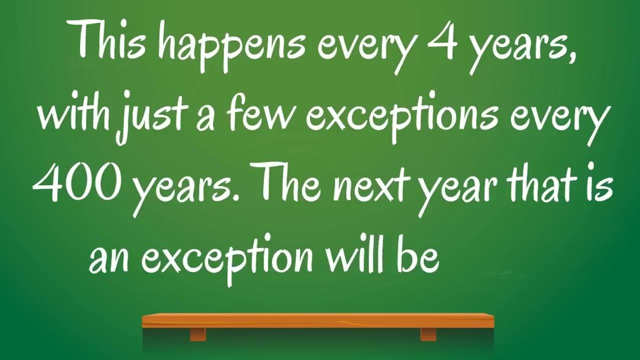 you actually have an extra day To fix this problem. we just add an extra day to February, called leap day, to equal everything out. This happens every 4 years, with a few exceptions every 400 years. The next year that is an exception will be the year 2100. 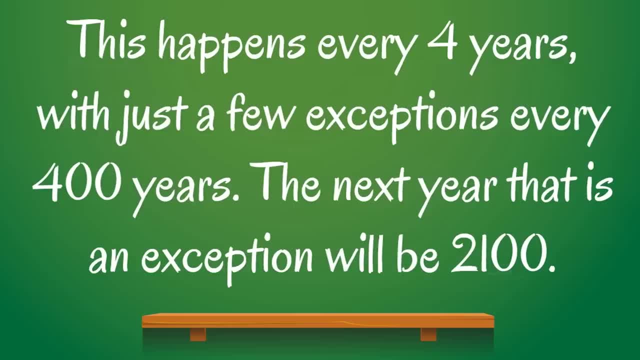 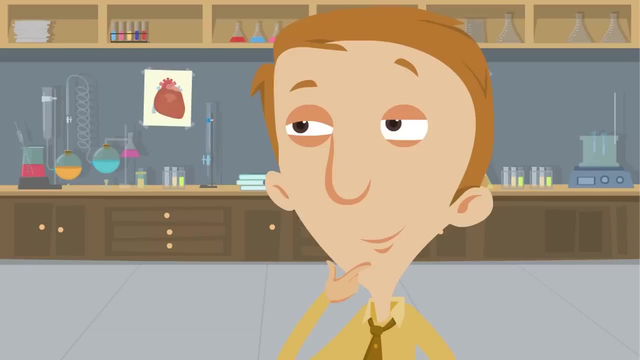 It will be a fourth year but will not have a leap day. What if someone from that year in the future is watching this video right now- Wow, that would be so cool, wouldn't it? Or if you are watching this as a kid. and in 2100, when everyone is looking forward to leap year. 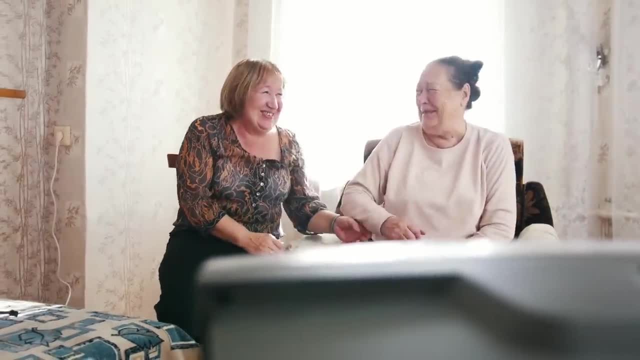 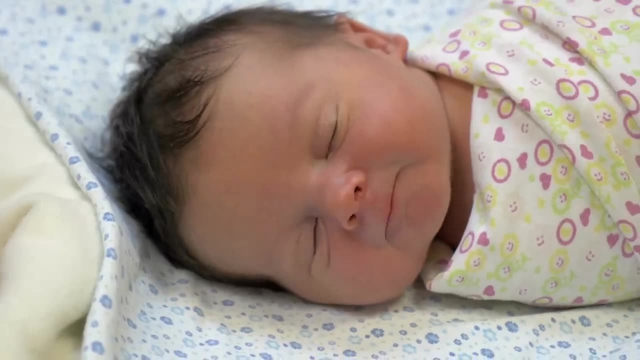 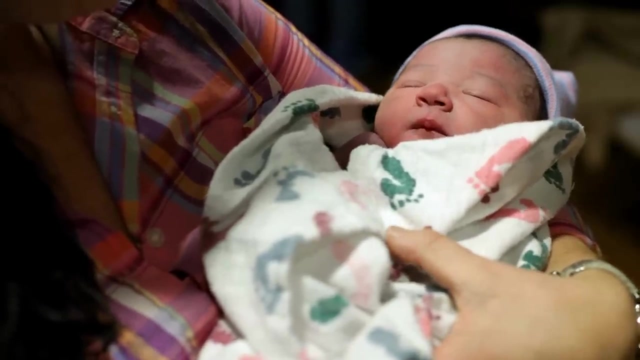 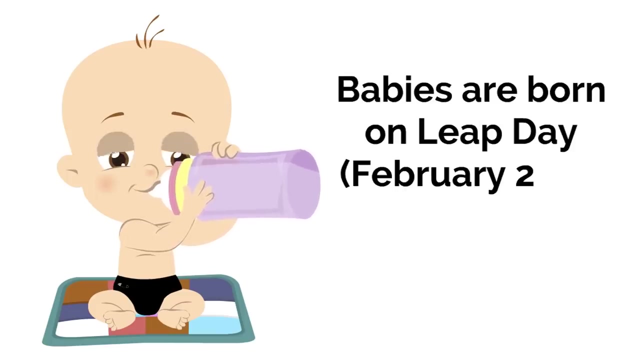 you'll say, hey, leap day isn't happening this year. I saw a Hope School Pop video about it a long time ago. Alright, Alright. The final fact has to do with babies. Oh, babies, Babies are born on leap day, February 29th, just like any other day.